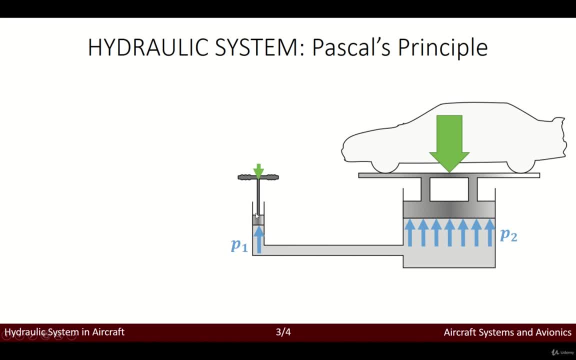 Right. so the main idea here is that we have this kind of u-tube- okay- over here which is connected by this fluid okay, which you can see in gray, right. so, as you probably know, a fluid has a relation to pressure, okay, meaning that any fluid that you know will be related to some amount of pressure, and this 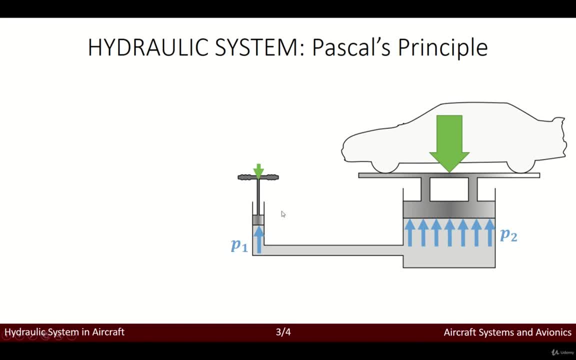 amount of pressure is, of course, exactly the same throughout all the fluid, right? so again, the meaning here is that by applying a certain amount of force, we would actually be providing or applying a certain amount of pressure to the fluid, and by applying another force- okay, over here. 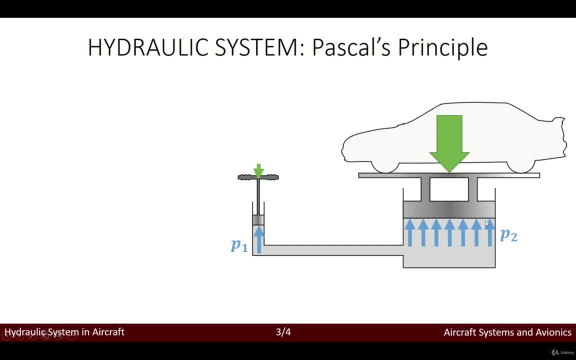 we would actually be providing another, you know another- pressure to the fluid over here and, as you can see, there's a certain continuum. okay, so basically, we have a pressure over here and a pressure over here. right, a hydraulic fluid is connecting two pistons, this one and this one. 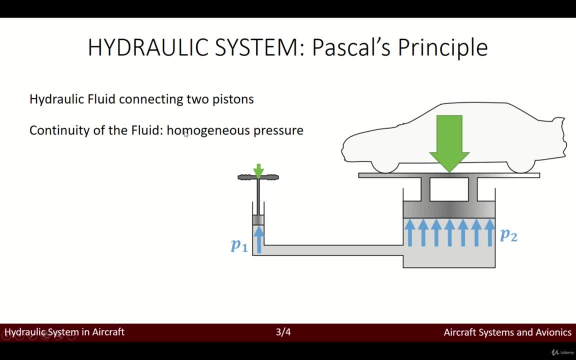 right And due to the continuity of the fluid, we will have an homogeneous pressure. What does this mean? The fact that, even if we here see that this is pressure 1 and pressure 2, we need to establish because of the continuity of the fluid. 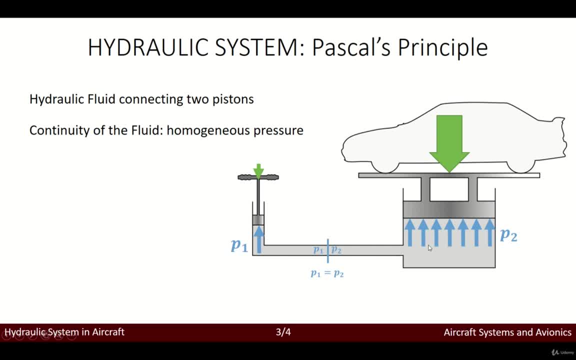 that all the pressure throughout the fluid will actually be the same, meaning that pressure 1 and pressure 2 will be the same, And this is what is known as Pascal's principle. Why is this important? Well, the fact is that the pressure is actually the relation between the force and the area it acts on. 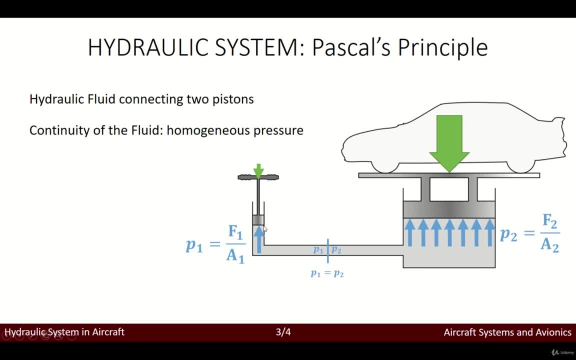 Meaning that this force divided by this area- suppose that this is cylindrical- is equal to this amount of pressure. And this amount of pressure is actually equal to this amount of force, which is the weight of the car, in this case, divided by the area. 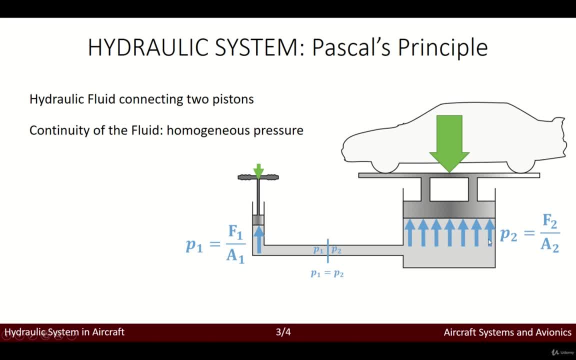 So, as you can easily see, derive, pressure 1 and pressure 2, are the same, as stated before. So force 1 divided by the area 1 is equal to force 2 divided by area 2.. Now the idea here is that we can actually lift the car with a tiny force. 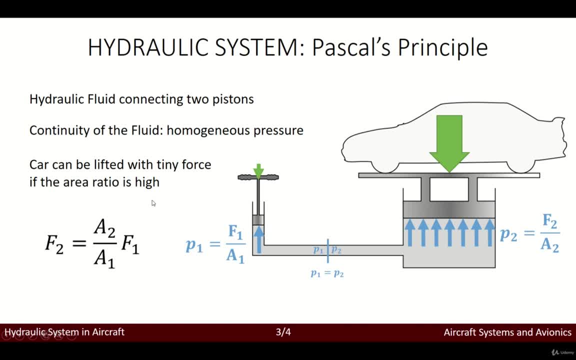 if the area ratio is high enough, Meaning that the relation between the force 2,, which is the weight of the car, and force 1,, which is the pressure or the force that we would be applying on this piston over here, is actually nothing else than the relation between the areas. 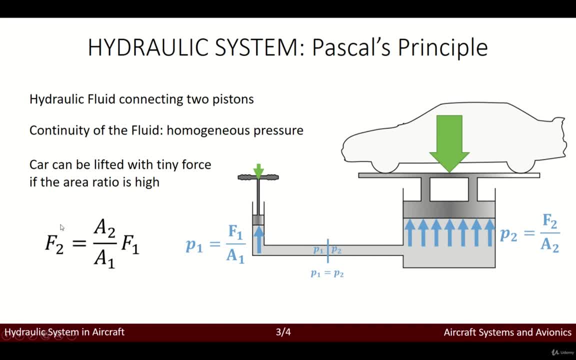 So, as you can see, imagine the car weighs- let's assume 1,000 kilograms And the force that we apply is 1 kilogram- Then, by simply deriving the ratio between areas, we can see that if this is 1 square meter, 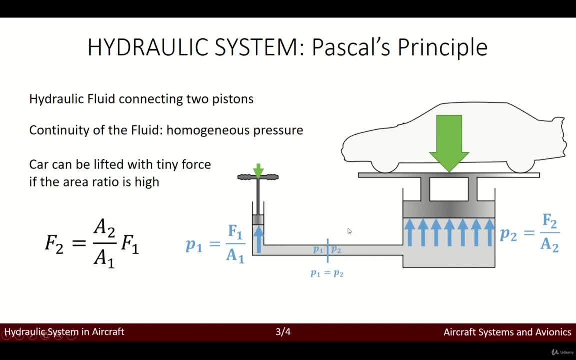 or let's put 1 square centimeter, we would actually we need 1,000 square centimeters over here- as to provide 1 kilogram of force over here and be able to lift a car which is 1,000 kilograms over here. 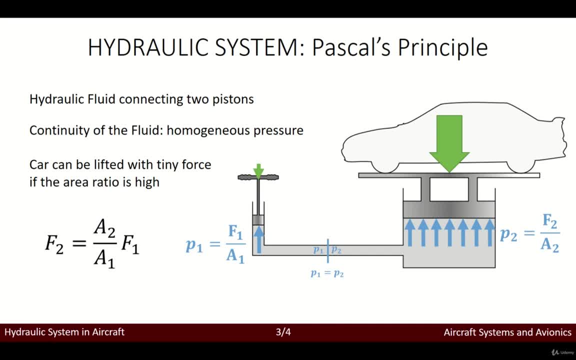 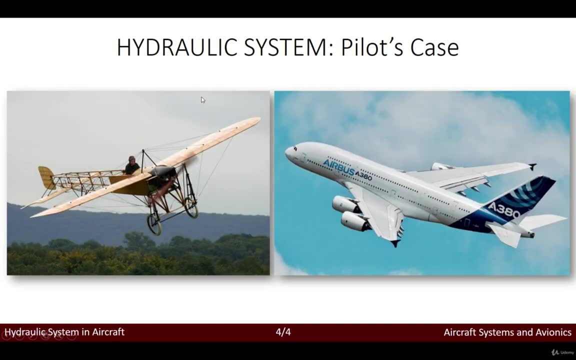 And this is actually very important in aircraft, Meaning that if the pilot does a relatively small force, we can actually be able to move big components on the aircraft through this kind of transmission- okay, Using hydraulic system, Right. So again, I just wanted to remark this, this idea. 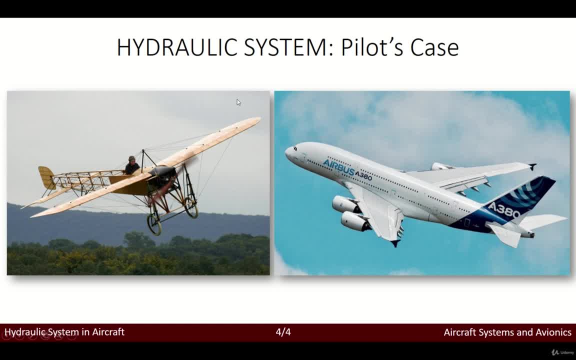 by having this as a bit of an example. The idea is that traditionally in aircraft, especially at the beginning, there was no transmission due to hydraulic systems. okay, The pilot would directly imply, you know, would make a force, and that force would be. 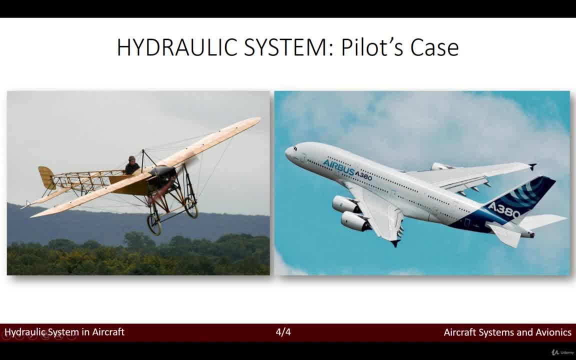 would provide actually the movement on the aircraft tail, for instance, on the different surfaces: control surfaces on the tail, okay, Or the ailerons on the wings. However, nowadays, as you can imagine, especially on the case of the Airbus A380,, 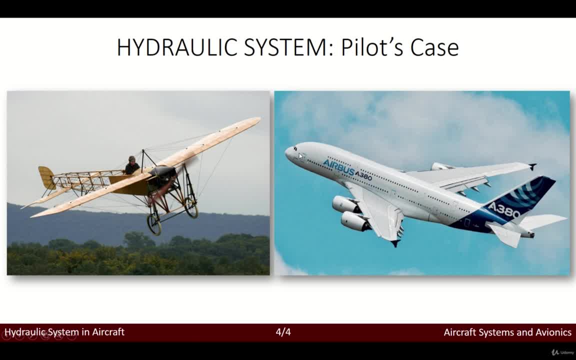 you can simply say: okay, there's no way that the pilot will be able to make that kind of effort in order to move the flaps, for instance, of the aircraft. Therefore, it's absolutely essential to have good hydraulic systems, and 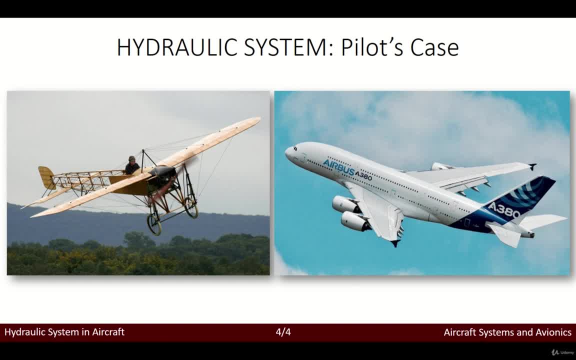 you know, to make sure that this system is reliable and functions correctly throughout the flight. okay, So with this we can go to the next class. Thank you.